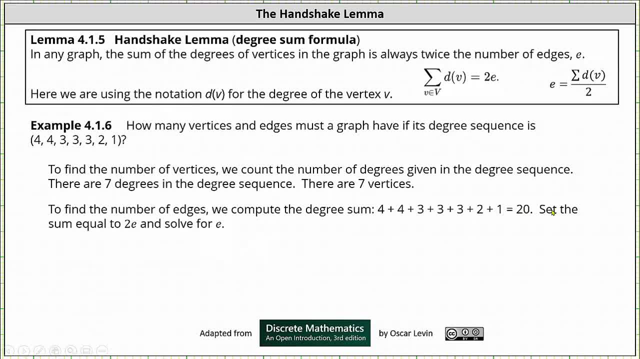 we compute the degree sum which we can see is equal to 20, and then we set this equal to two e and solve for e. This gives us the equation two equals 20,. dividing both sides by two, we have e equals 10.. 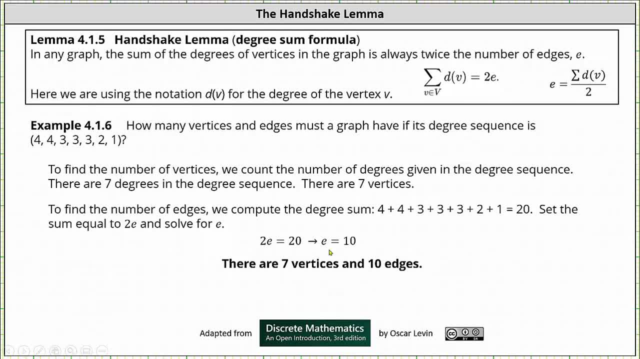 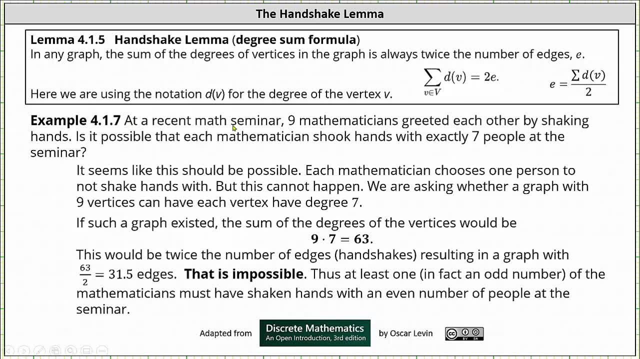 We now know, the graph must have seven vertices and 10 edges. The Handshake Lemma also tells us what is not possible. As an example, at a recent math seminar, nine mathematicians greeted each other by shaking hands. Is it possible that each mathematician shook hands? 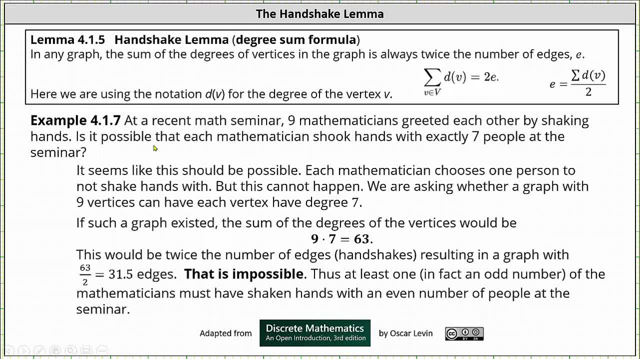 with exactly seven people. at the seminar, It seemed like this should be possible. Each mathematician chooses one person to not shake hands with, but this cannot happen. We are asking whether a graph with nine vertices can have each vertex with degree seven. 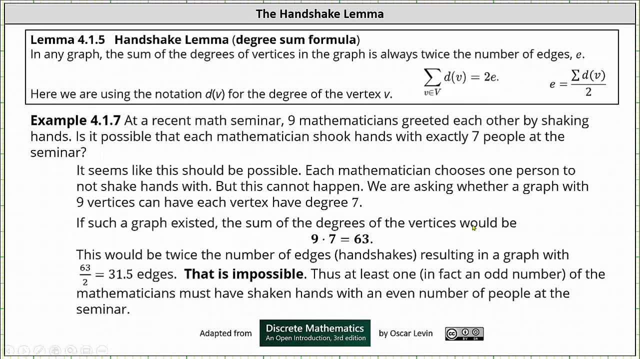 If such a graph existed, then the sum of the degrees of the vertices would have to be nine times seven, which is equal to 63.. This would need to be twice the number of edges or, in this application, the number of handshakes. 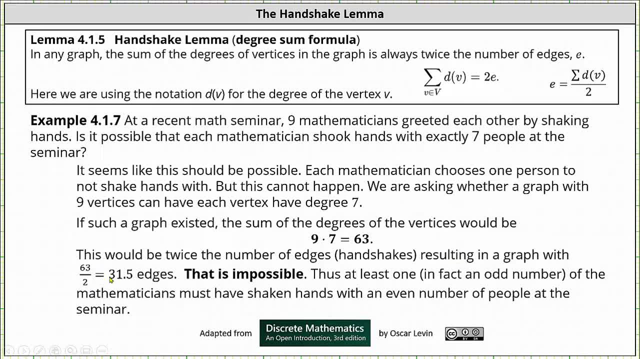 resulting in a graph with 63 divided by two or 31.5 edges. But we know, the number of edges has to be a whole number and therefore that is impossible. Thus at least one, in fact an odd number of the mathematicians must have shaken hands. 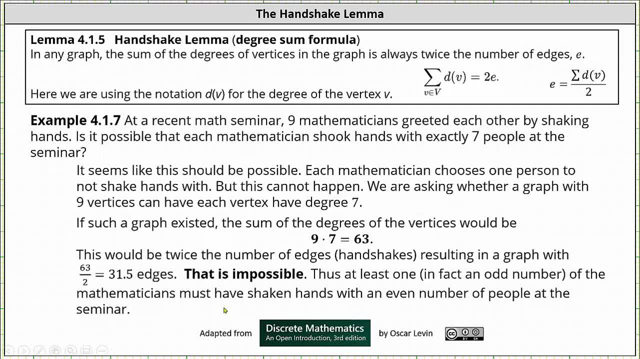 with an even number of people at the seminar. And this is because, as we know from the first example, the sum of the degrees sequence must be even in order for the number of edges to be a whole number. We generalized the previous example to get the following proposition: 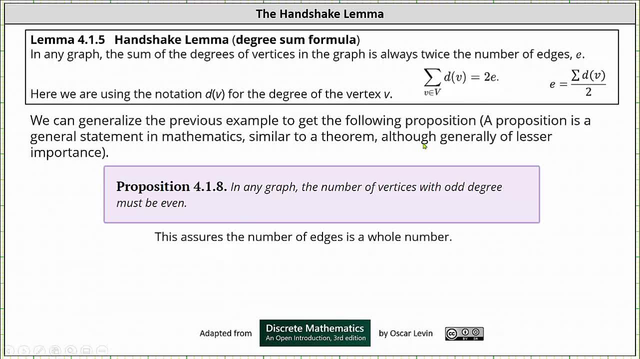 A proposition is a general statement in mathematics, similar to a theorem, although generally of lesser importance. The proposition is: in any graph, the number of vertices with an odd degree must be even. This assures the sum of the degrees is even and therefore the number of edges is a whole number. 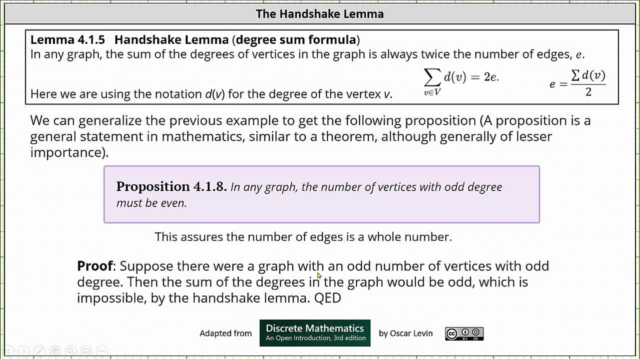 And we'll end with a quick proof of this proposition. Suppose there were a graph with an odd number of vertices with odd degree. Then the sum of the degrees in the graph would be odd, which is impossible by the handshake lemma. I hope you found this helpful. Thank you. 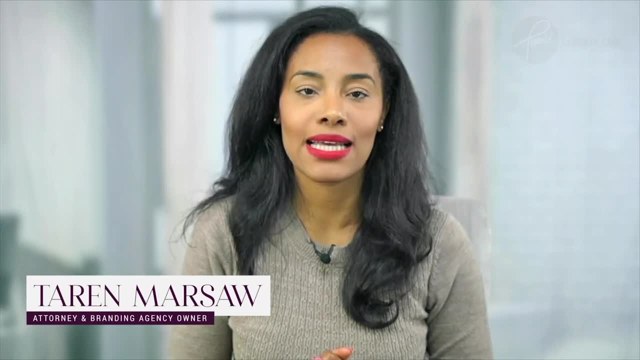 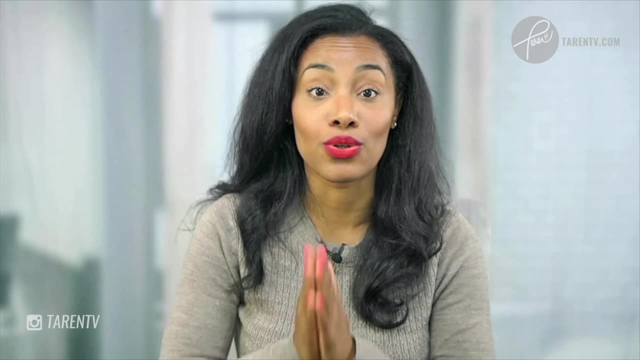 Hey guys, we're talking about the trademark application preparation process. Ooh, say that twice: If you're ready to pursue a trademark, you will want to prepare some documents. Even if you are going to use a lawyer, you'll want to kind of come prepared, And I'm going to.